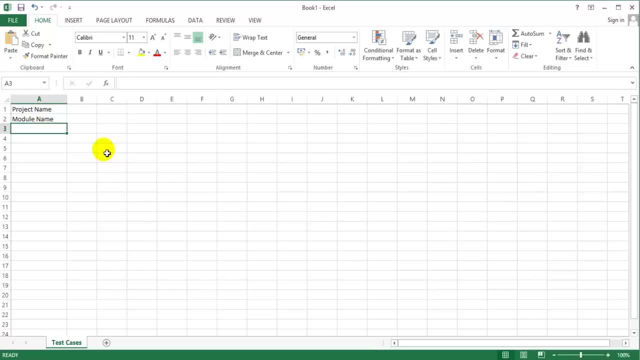 case, And once the test case is created, someone should review the test case, either by the peers or by a team lead. So the first thing we need to do is to create a test case template. We need to add a field: reviewed by and reviewed date. 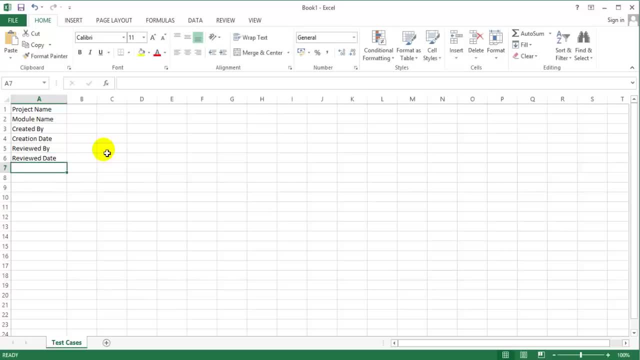 So we are going to take the next field as test scenario. Here our test scenario based, our requirement is verify the login functionality of a Facebook login page, So we need to take a test scenario description. So for each and every test scenario we write test cases. So I am going to take a test case id. 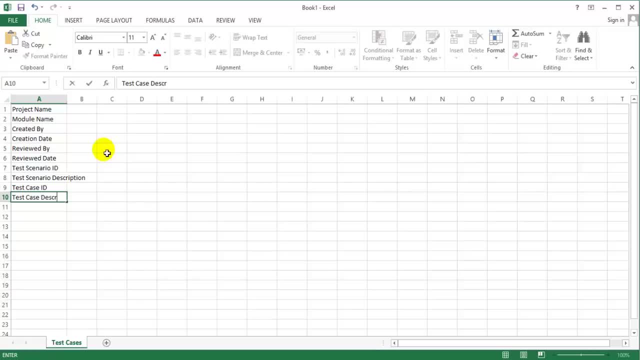 and test case description. For every test scenario there will be a pre conditions and post conditions. Imagine, for the login functionality. to verify the login functionality, the pre condition here is we need to have a valid URL, And for the post condition, after the login it will show either a post page or some your 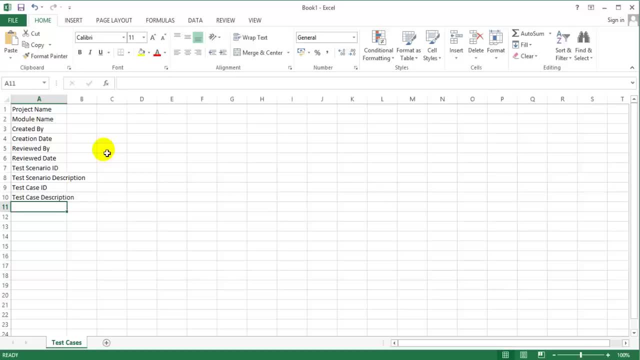 favorites page, something else based upon the application, the relevant landing page will display So the pre conditions and post conditions we need to take. So, after pre conditions and post conditions, after to execute a test scenario, we have to assume a expected result and actual result. So we have to take expected result field and actual result field. 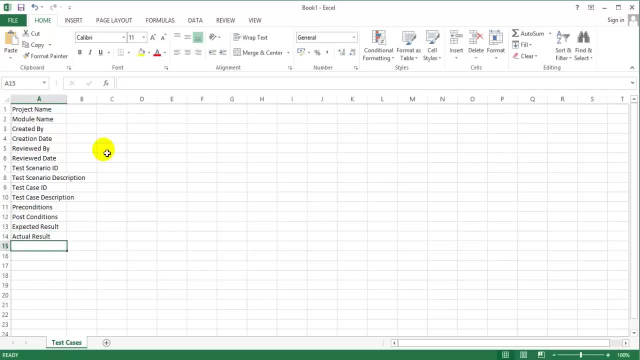 And we need to take a status because after executing the test case, we need to see the status, whether it is pass or failed. So earlier we have taken who created this test case and who reviewed this test case And while executing the test case, someone will execute the test case. 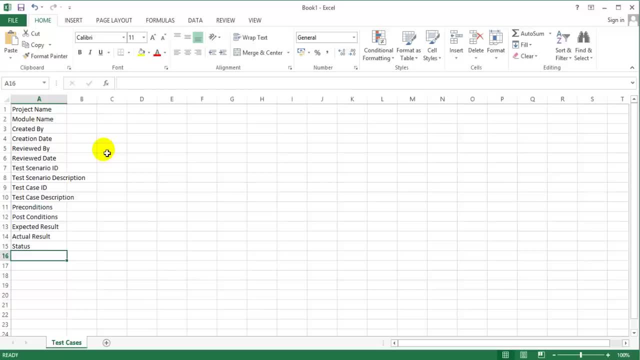 So we need to take the name of the tester here. So we need to take another field as test case: executed by and executed date, which means when the tester executed the test case, And comments, if any. So let's reorder the fields In the template. for each and every template, we need to have a project name, module name. 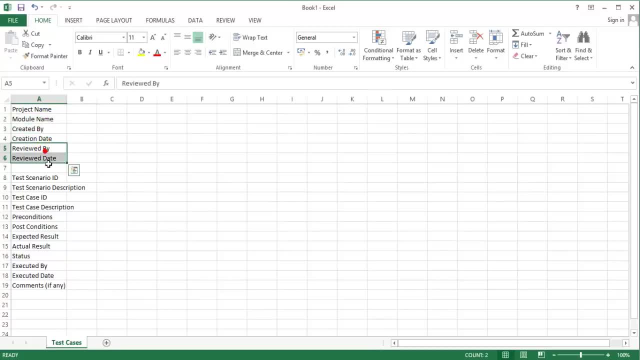 created by. created date. reviewed by and reviewed date. So, and these fields, I'm going to keep it as a horizontal way. So what we will do is we are going to take and edit the project name. I'm just going to do the all header by inside element targeting. 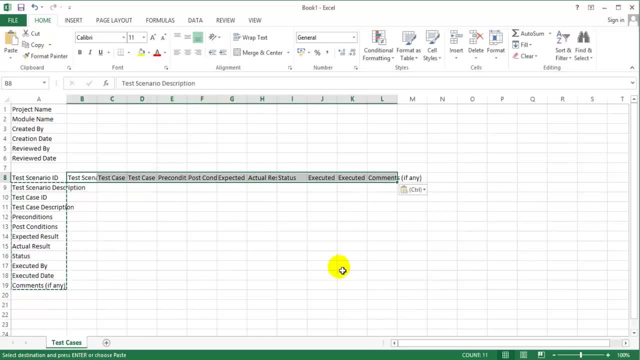 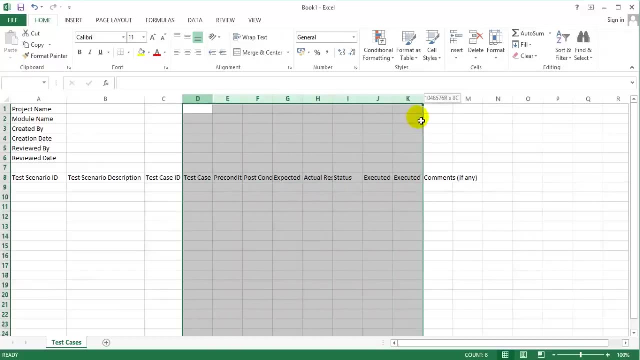 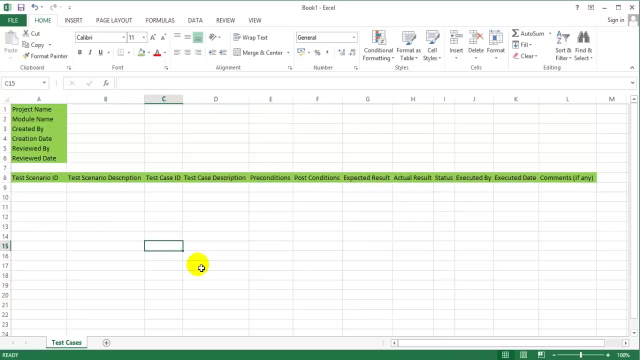 And then if there is a dot, these blocks are what we're going to do. So again, I started already offered to do this, Sorry. So we take or see. So what p? e we take or see, I am going to take a project name as Facebook and the module name as Facebook login page. 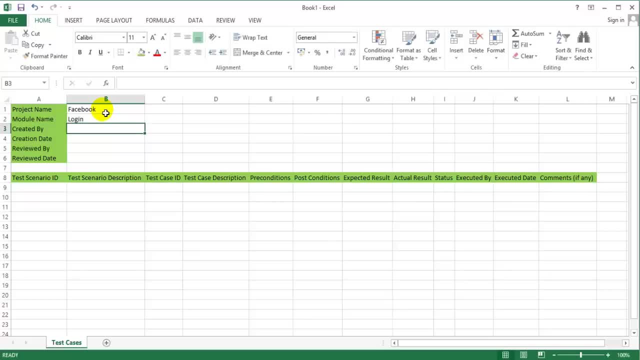 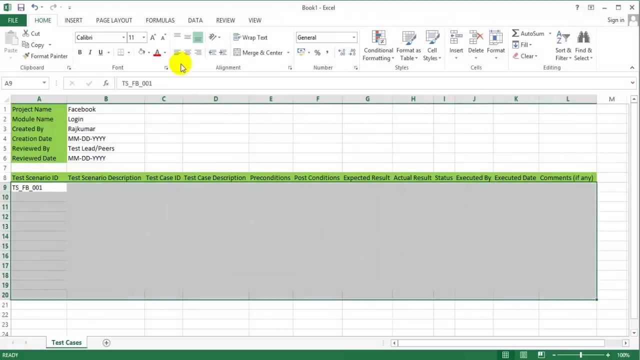 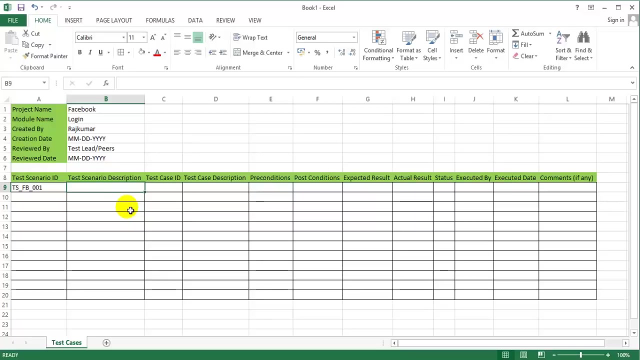 so login and created by and creation date or out the date you went and review by test lead or any peers review date and my test scenario ID is DS 0 0 1 and the test scenario description verify the login functionality of Facebook login page and for this functionality, for this test scenario, I'm 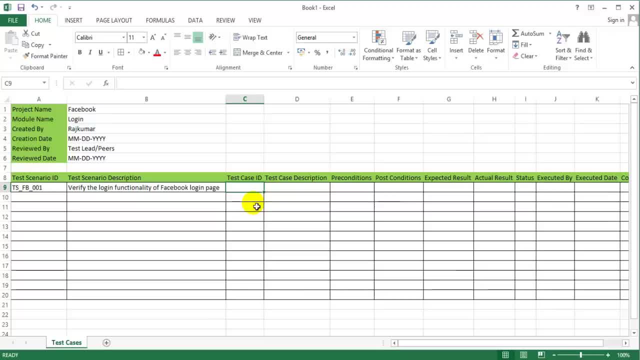 going to write a test cases. I'm going to take a test case ID. do you see? we log in 0, 0, 1 and the first test case description is a positive test case. enter a valid username and valid password and click on login, set password and send new Bedo. 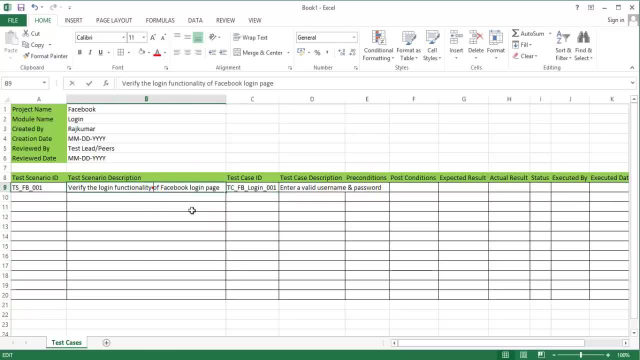 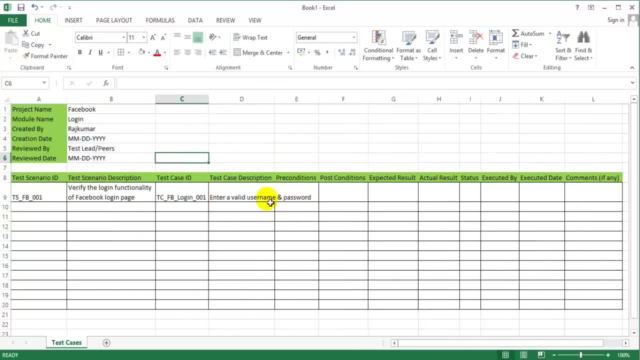 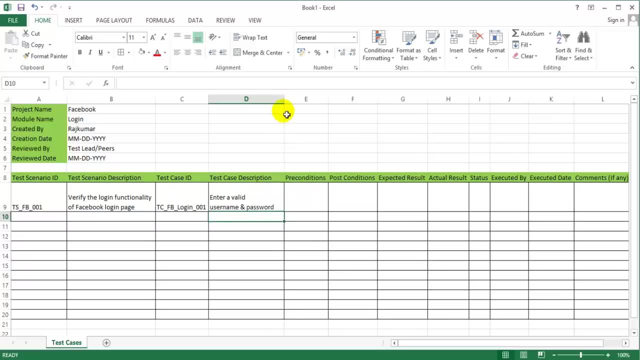 satisfies. this continues before going to see the conditions and poor condition. let me take써 other test cases too, and my next test case is the test case ID is test case number two and so on. like I'm going to take two more test case IDs, 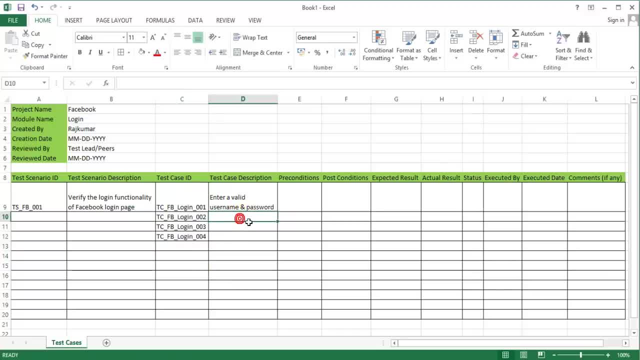 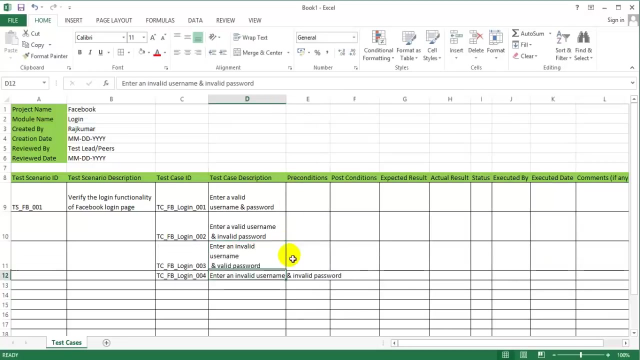 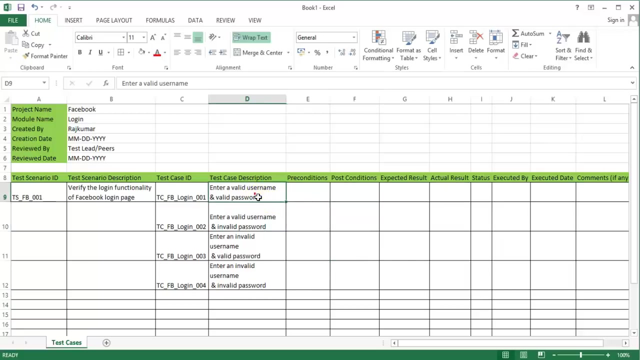 you enter a valid user name and invalid password and enter valid, enter an invalid user name and valid password and finally enter an invalid user name and invalid password. okay, fine, now I'm going to segregated the test case into test steps, so I'm taking one more test case out of digit zero, so let me delete it. now I'm going to take two New. 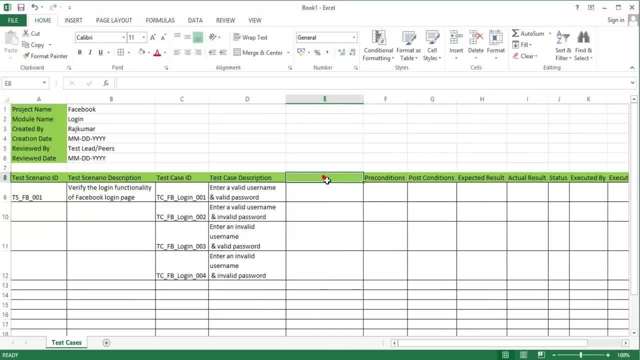 field here as test steps. here I will write step one, step two, step three for each and every test case. so my first step is for the positive test case, this, this one is a positive test case and these three are negative test cases. now writing the test steps. first step is enter valid username. enter valid. 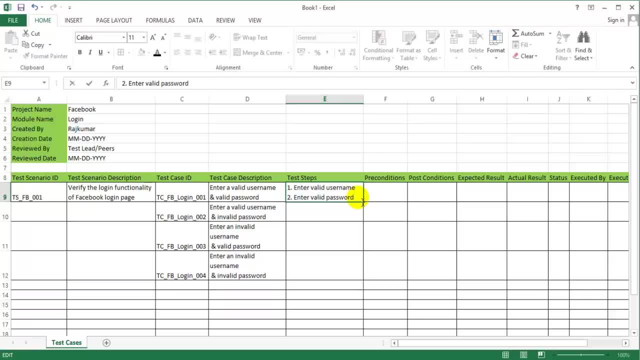 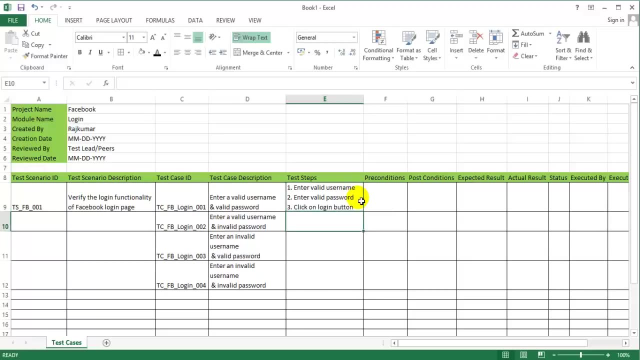 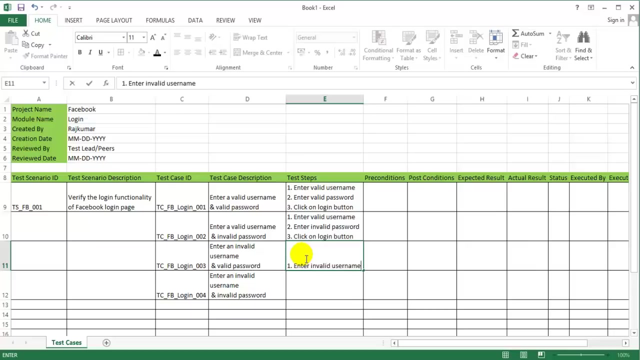 password enter. click on login button. and for the second test case, my test steps are: enter valid username. enter invalid password. click on login button. and test steps for third test case: enter invalid username. enter valid password. click on login button. and finally, for the fourth test case: enter invalid. 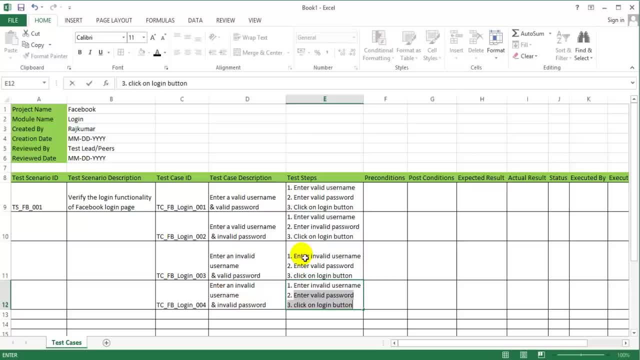 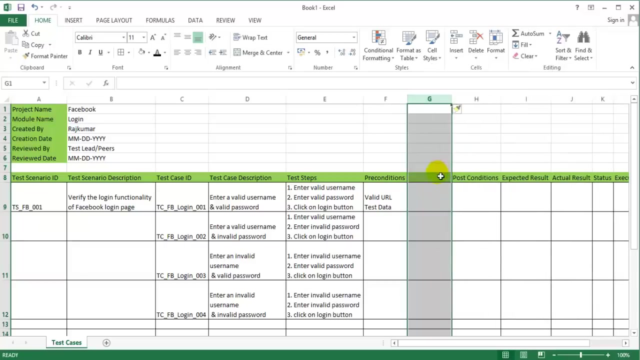 username, enter invalid password and click on login button. so for these test cases, the preconditions are: we need to have a valid username, so valid you are, test data and so on. like you, now let's add one more field as test data for each and every test step, we 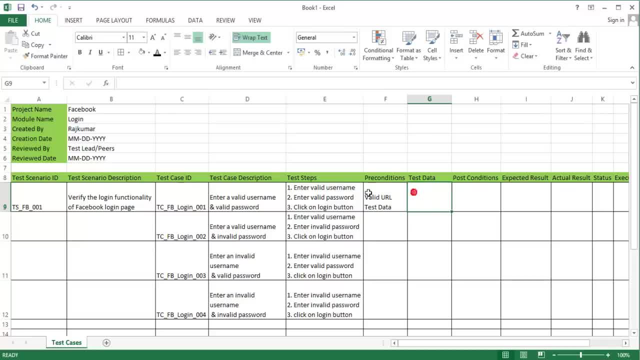 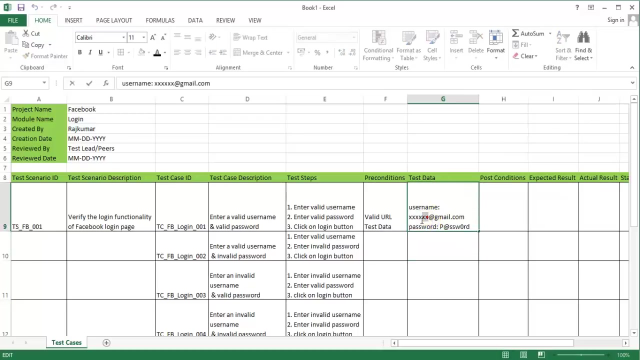 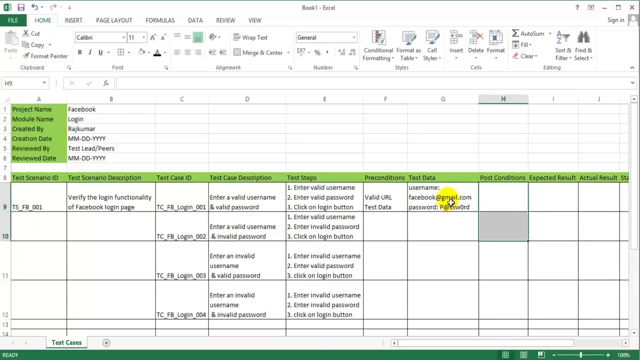 need to take a test data for each and every test step. we need to take a test data Here for enter: valid username and valid password. we need to have a valid username and valid password. These are the valid username and password. is my test data. and for the second test case: 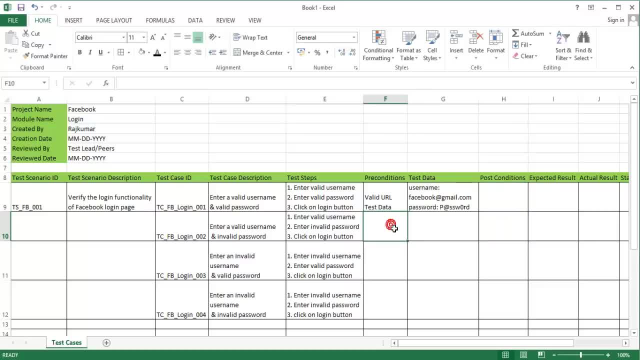 the preconditions are the same preconditions for all the test cases, because all the test cases are similar powers and for all these test cases our test scenario is same and test description is same. so I'm going to copy and paste here. so for the second test case, my 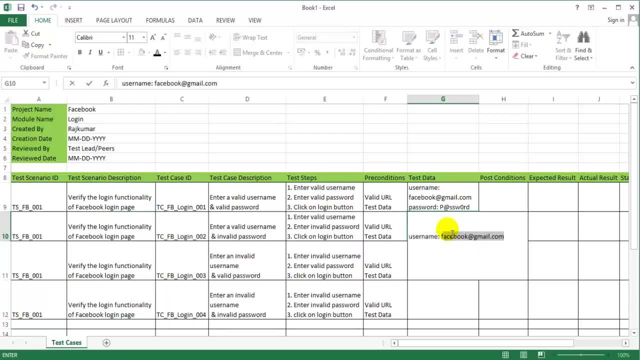 username should be valid. why? because, based upon the test step, the username is valid and the password is not valid. not valid, it's an invalid password. actually, we are going to take an invalid password to make the test case fail. similarly, I'm going to take a user name for the. 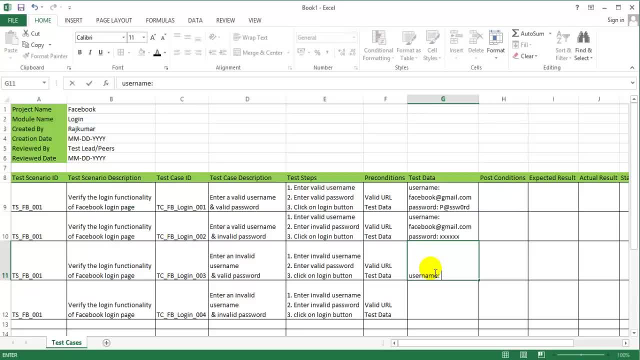 third test case as invalid test case. in my invalid user name here and password is valid one. see here. I took the test step one as enter invalid username and the valid password. so I took a invalid username and valid password and in the final test case the username and password are invalid. 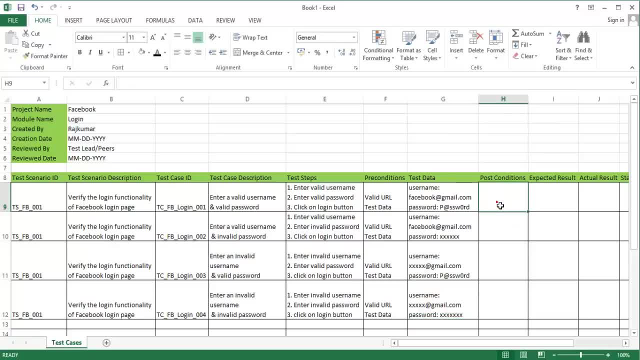 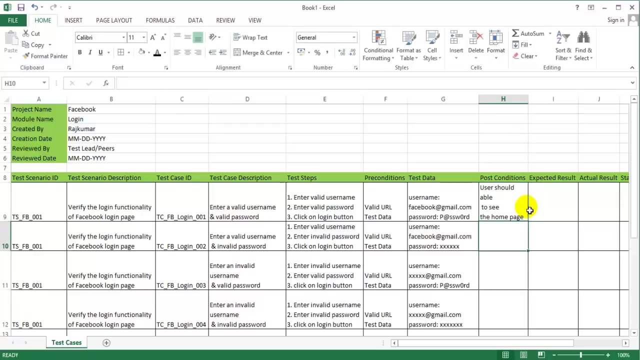 let's see the post conditions. the post condition here is: once I enter a valid username and valid password and click on the log login page, I need to see my Facebook main page. the post condition here is the user should able to see the home page. the expected condition here is successful login. we can see the actual. 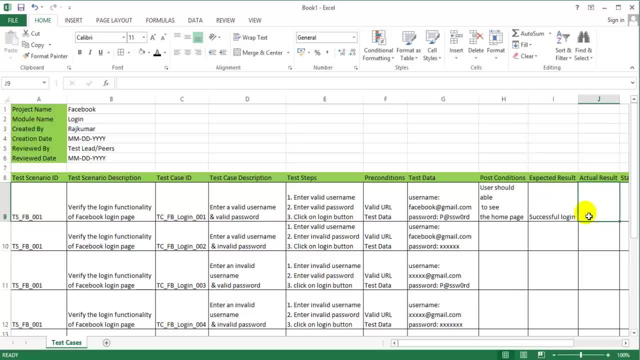 actual result once we executed this test case. for the second test case, the post condition will be a message pop-up from the Facebook login page as your username or password or invalid password in WhatsApp. this is the default experience for the Facebook email and you need to keep the default user profile for the Facebook account. 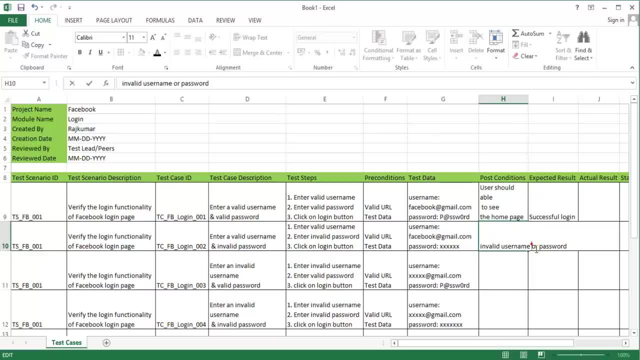 and you need to keep the default user profile for the Facebook account. so what we did? we? we did a right click, download and pull out our Facebook account and we will see the default user profile. here, as an example, I will show the default user profile and we can see the actual. 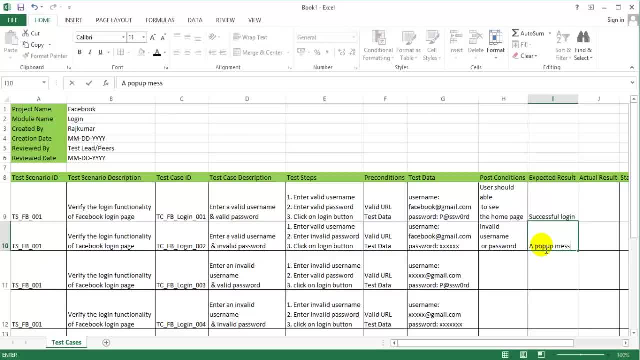 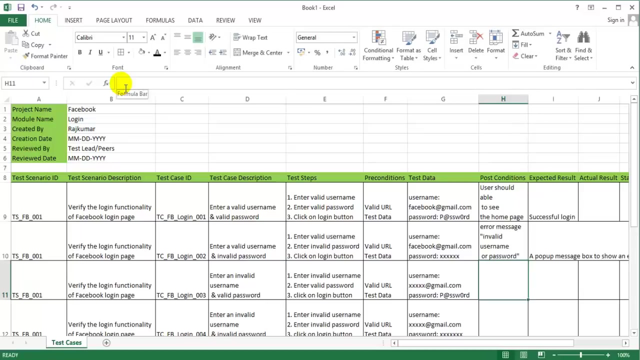 account. here A popup message box to show an error- that invalid username or invalid password. The popup message box to show an error- that invalid username or invalid password. Similarly the same way. here we are going to make the invalid username and valid password. So the post condition is same and for the final test case also the post condition will. 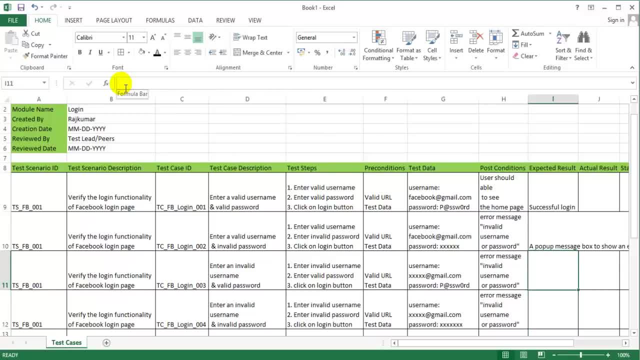 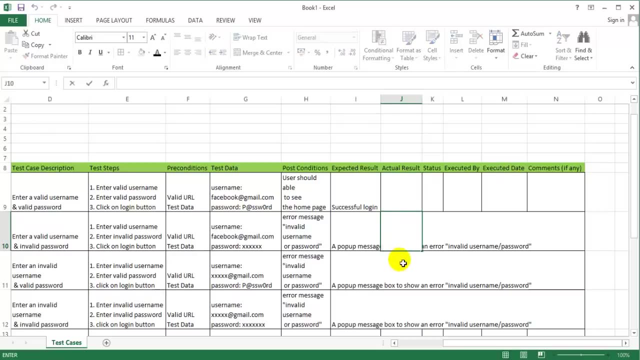 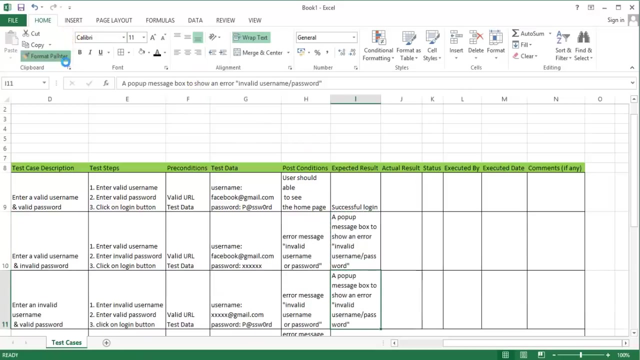 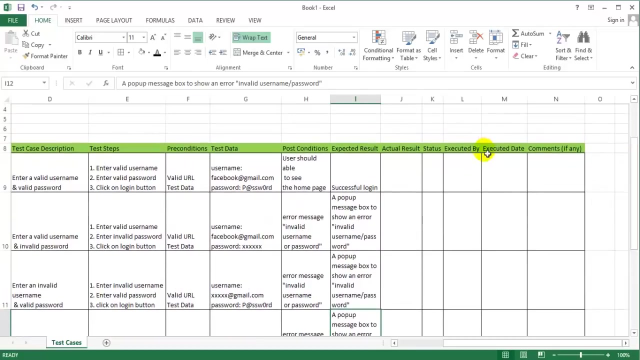 be same. So the expected result is same for the test case 3 and test case 4.. So once we execute these test cases, we can see the actual results. We can see the actual results And if the actual result and expected result are same, we make the status as pass, else we 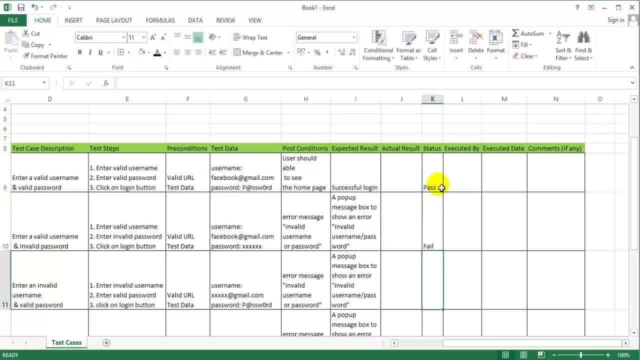 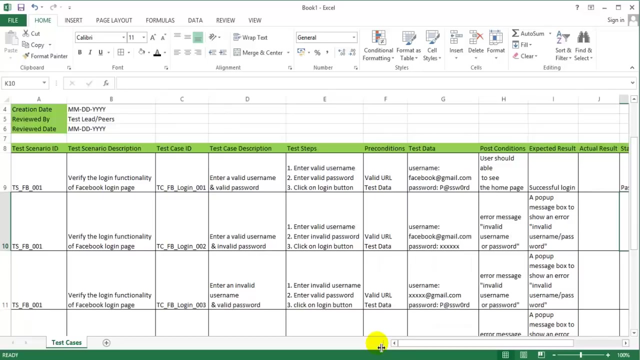 will make it false And we need to. the one who is going to execute the test case. he needs to add his name here, or employee id And executed it, And comments, if any. Likewise, we can fill each and every field here. This is the way we are going to create a test cases for every requirement.